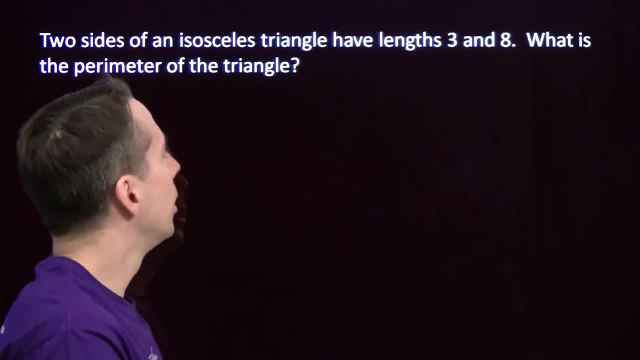 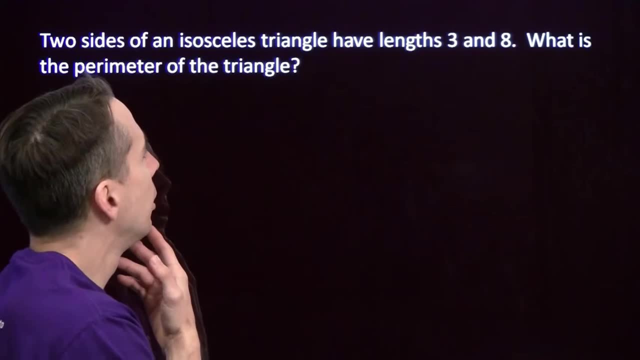 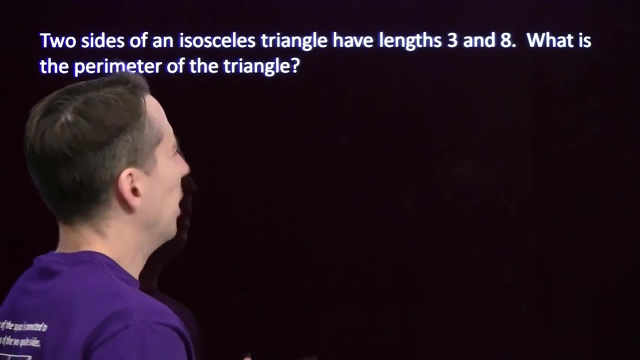 the triangle is isosceles and these two aren't the sides with the same lengths. we know that the third side length has to be either 3 or 8.. We're going to make the triangle isosceles. Which is it? I can't tell. I mean, maybe there are two answers to this problem. Maybe. 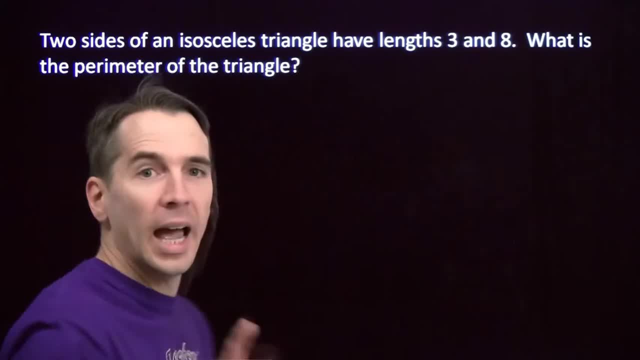 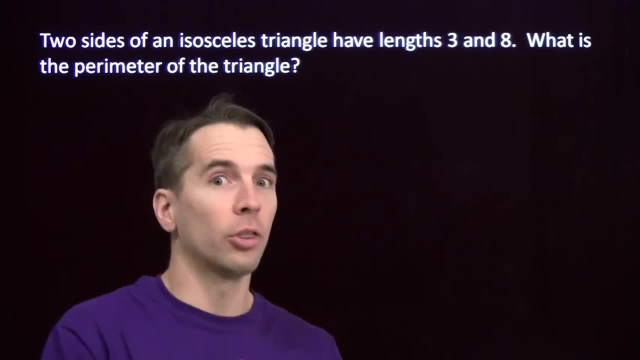 the problem's messed up. I have an idea. Here's what we'll do. We'll build two triangles. We'll build both possibilities. We'll build one triangle with side lengths 3,, 8, and 8.. And we'll build another triangle with side lengths 3,, 3, and 8.. Now, we'll take those. 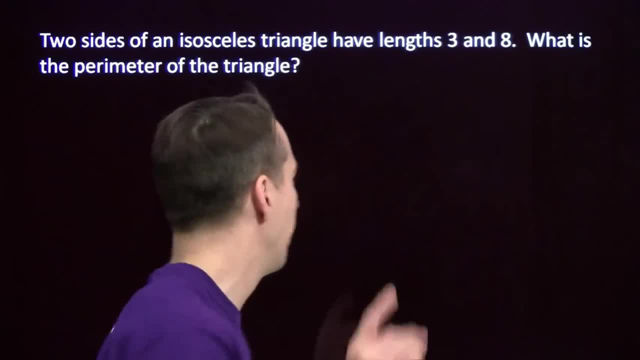 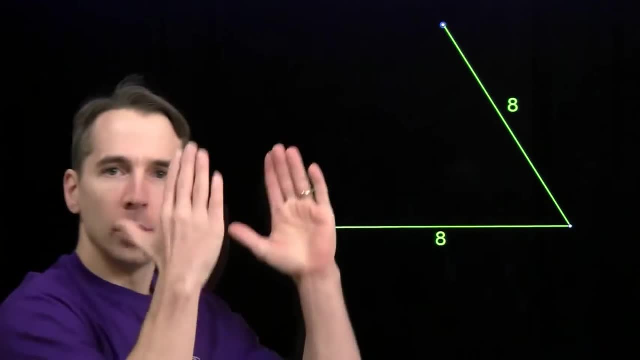 two triangles and send it to whoever made this problem and show them that they messed up. Here we go. We'll start with the 8,, 8, and 3.. So here are our three sides: 8,, 8, and 3.. And if I can just get these two ends to meet, we'll form a triangle. So let's just 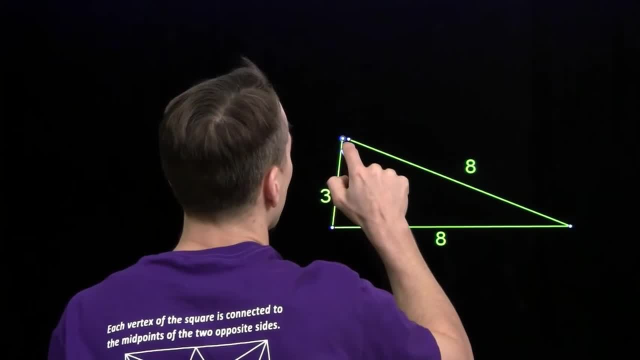 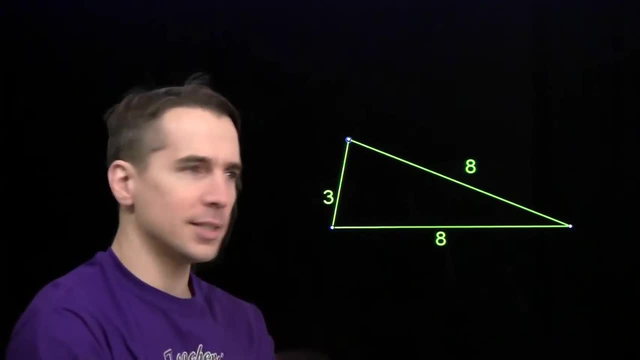 drag this down Here like that, Drag this over here, And there we go. We've got a triangle side lengths 8,, 8, and 3.. So that's one of our triangles to send to that person who wrote that problem. 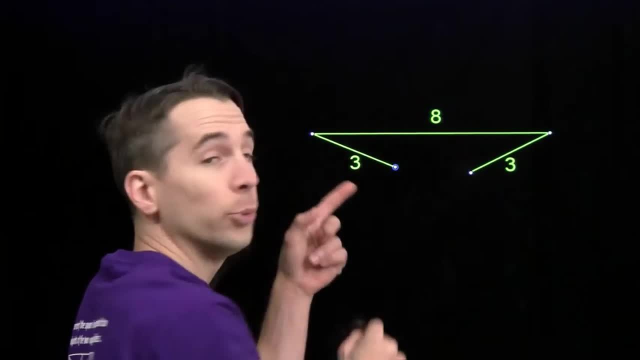 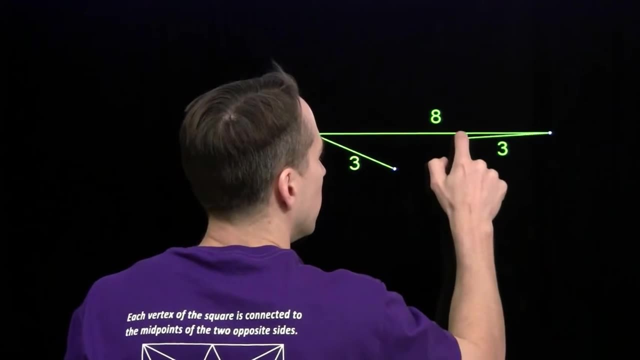 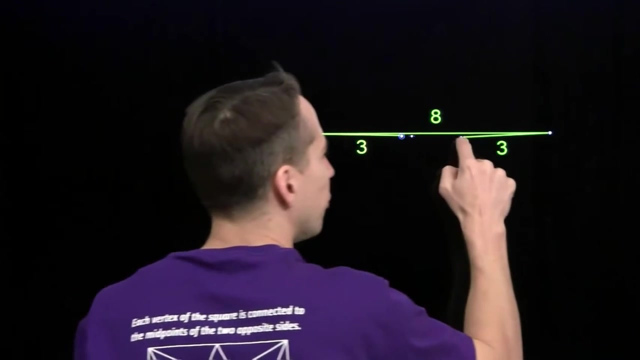 that's messed up. Let's build another one. We've got the side lengths 8,, 3, and 3.. Now, if we can just drag these around, get these ends, I don't think I can do it. I mean, if I put this one going this way as far as it can. 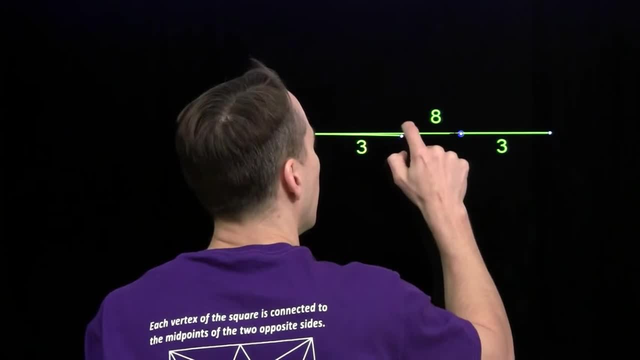 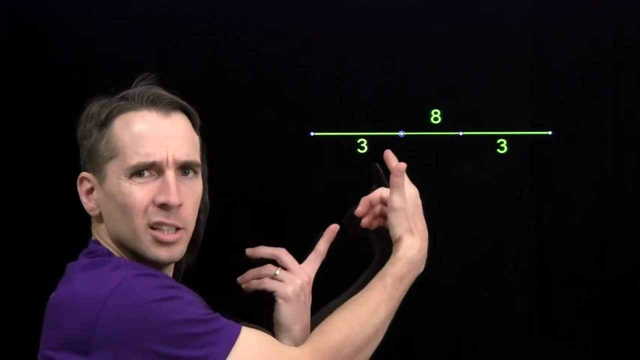 go and this one going to left. as far as it can go, still it's no good. I can go 3 in that direction from here, 3 in that direction from here, but that adds up to 6,, not 8.. They're. 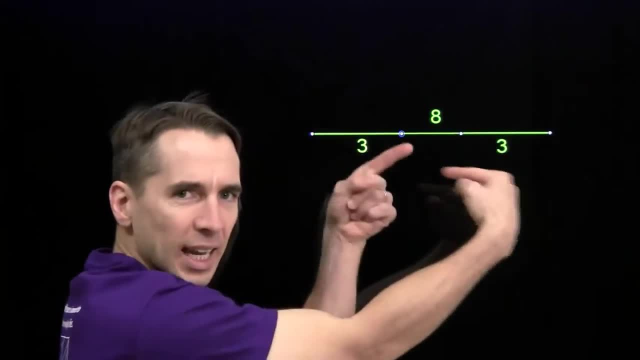 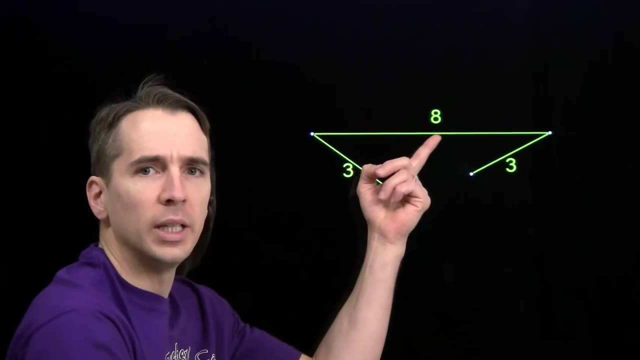 not long enough to reach. I need these two sides to add up to be at least 8 to be able to reach each other. I can't make a triangle with side lengths 3,, 3, and 8.. That means this problem isn't messed up. 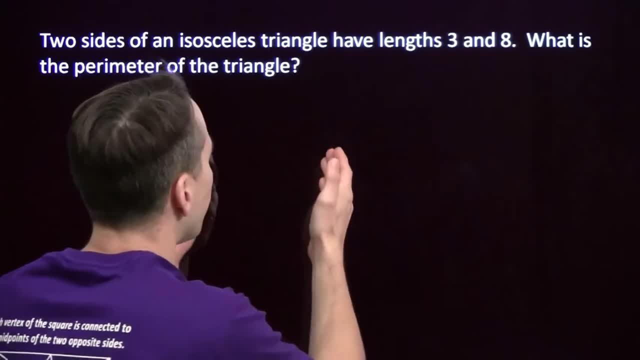 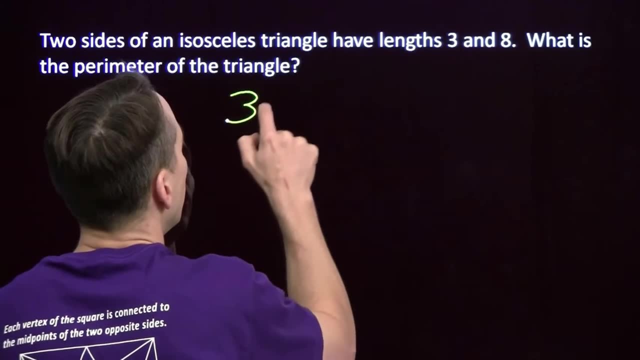 And this problem isn't messed up. And this problem isn't messed up. And this problem: the triangle side lengths are 3 and 8.. The third one has to be 8, because we can't make a triangle with side lengths 3,, 3, and 8.. So we can find the perimeter. 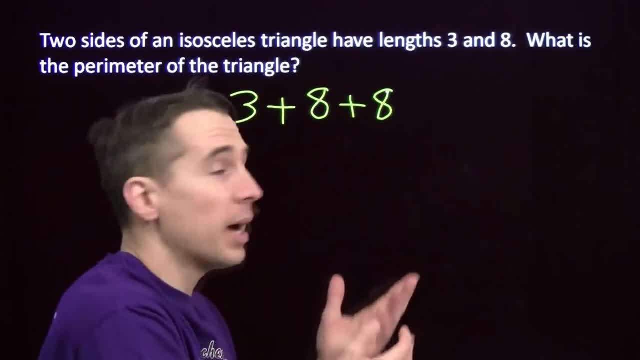 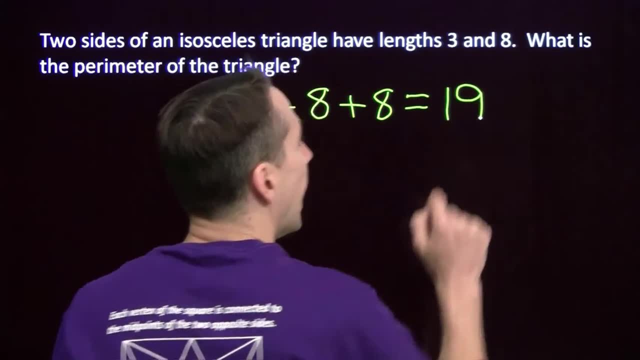 The perimeter is 3 plus 8 plus 8, because that's the only possibility. Two sides are 3 and 8, and the triangle is isosceles. We add these up. 3 and 8 is 11.. Add another 8.. 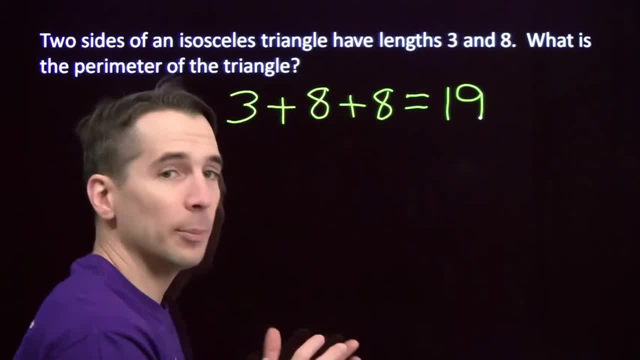 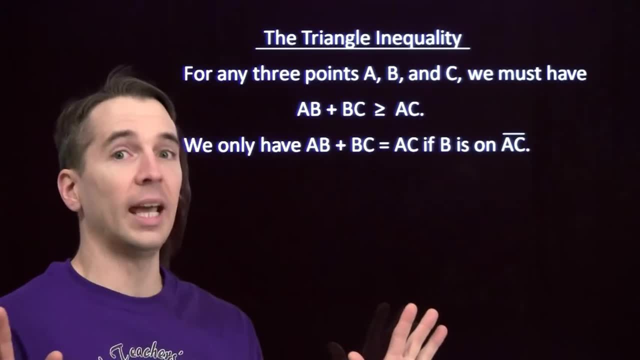 We get 19.. Now this problem is an example of a very powerful property in math. It's called the triangle inequality. Looks like it's about geometry, but you're going to see this again and again as you continue your studies of math. 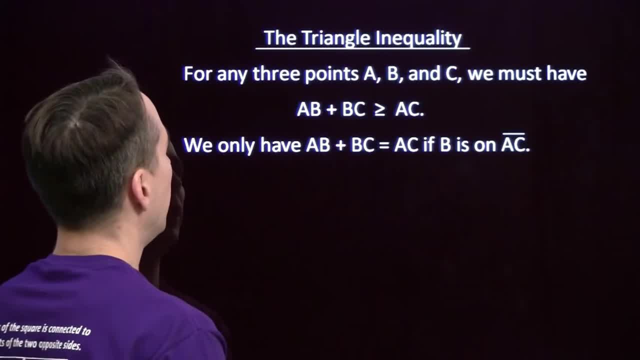 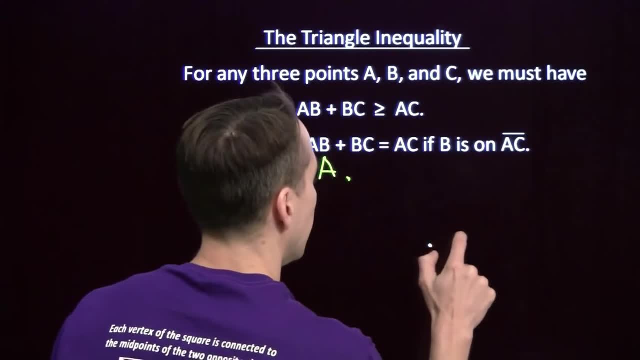 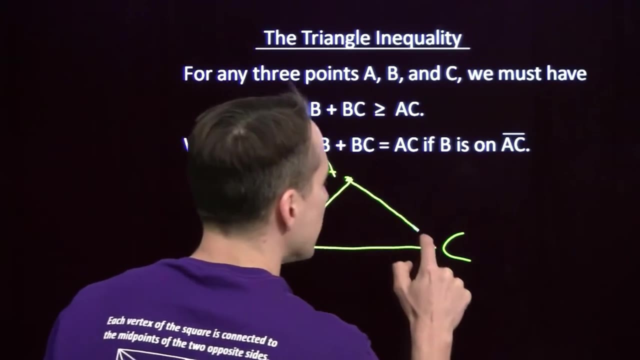 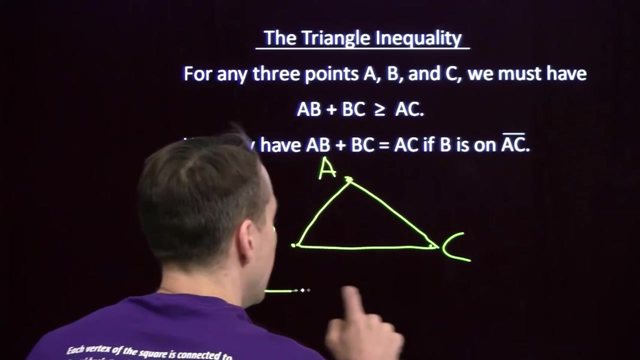 It pops up in all sorts of surprising places And here's what it says. It says: if you start off with any three points- A, B and C- then AB plus BC is always at least AC. The only way they can be equal to this sum, AB plus BC can equal AC, is if all three points. 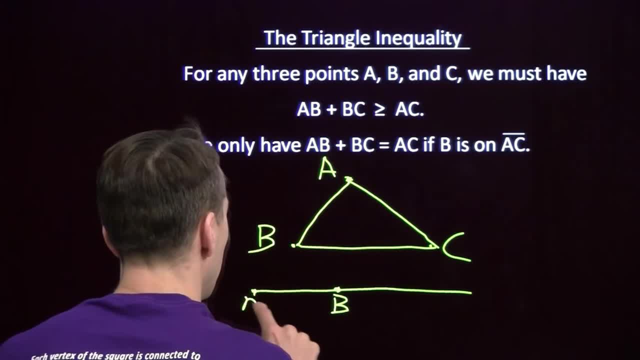 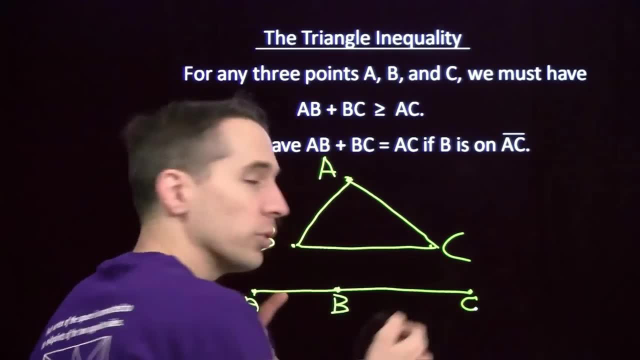 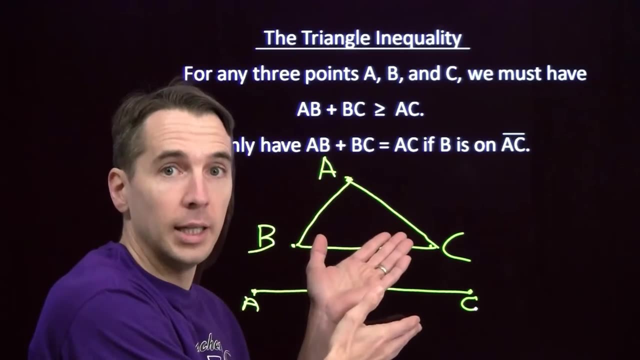 are on the same line and B is between A and C, In other words B is on segment AC, then here we obviously have: AB plus BC equals AC. But if B isn't on segment AC, like up here, then AB plus BC is greater than AC. 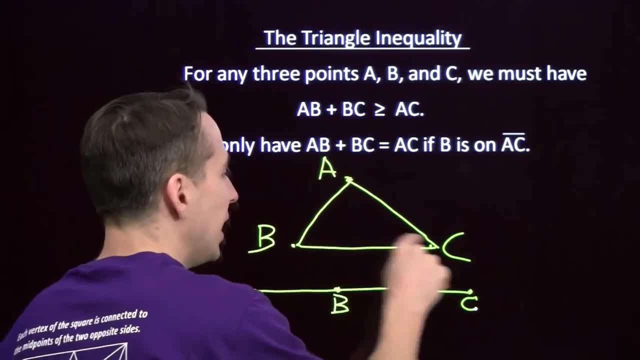 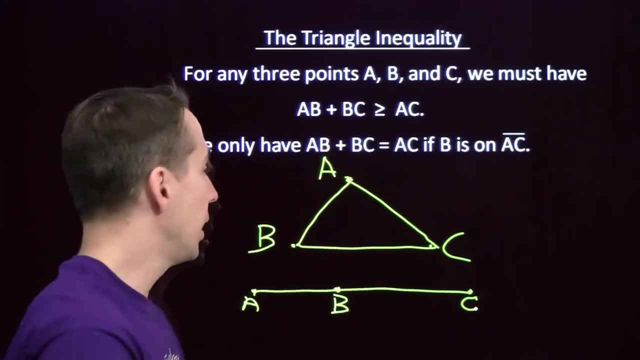 And what that means is: in any triangle, the sum of any two sides is greater than the third side. AB plus BC is greater than AC. AC plus CB is greater than AB. BA plus AC is greater than BC. Any triangle, this is true. 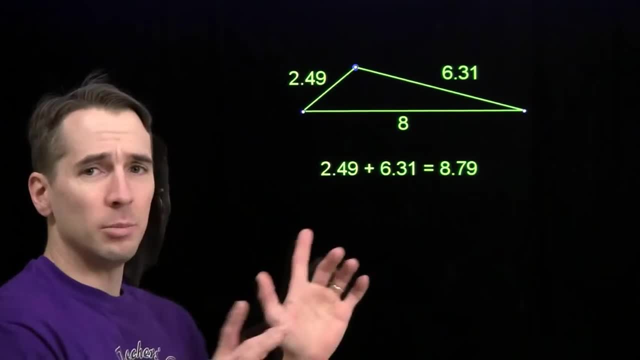 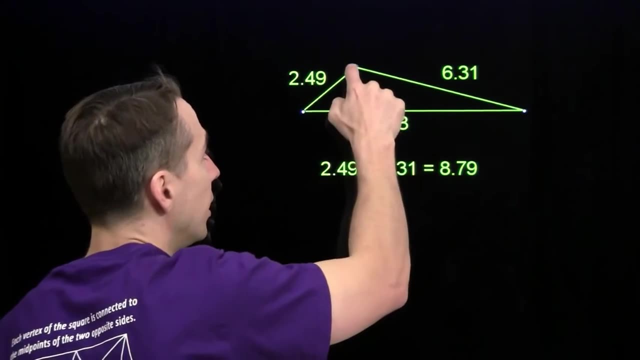 Had two sides, it's going to be greater than the third Seemed a little fishy to me so I checked it out, Built this triangle. This side length is 8.. Now watch what happens to the sum of the other two sides as I drag this point around. 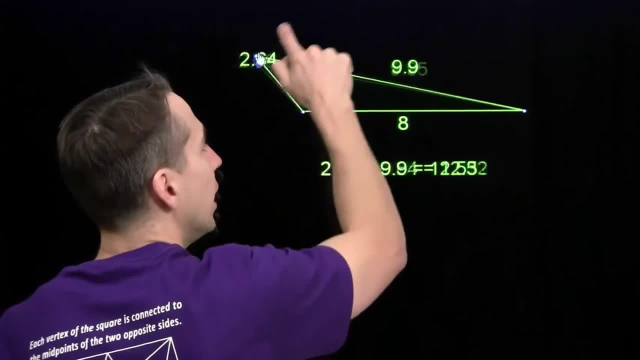 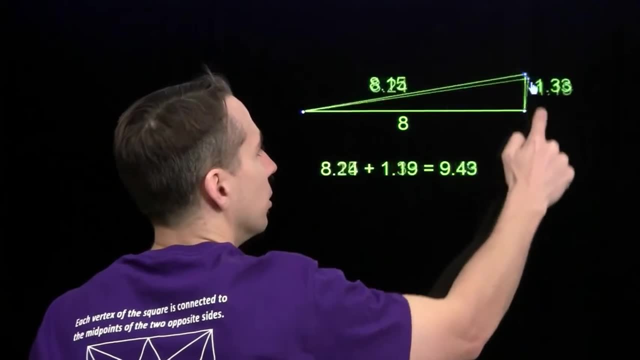 Drag it all over the place, It's always greater than 8, unless I put it boom right on 8. on that line I can make it equal 8, I can't ever get it less than 8.. Always at least 8, and if I have a triangle it's greater than 8.. 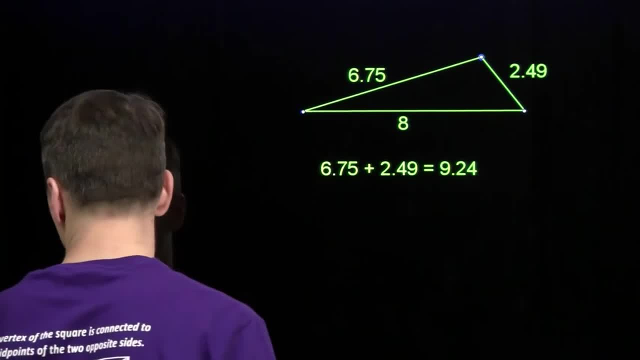 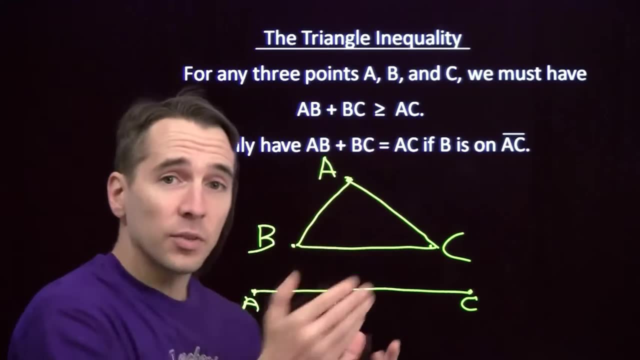 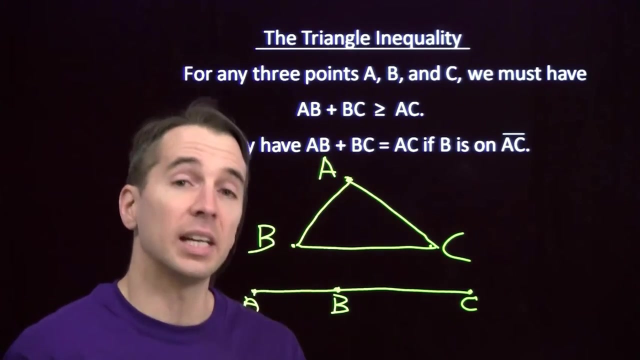 That's the triangle inequality. That's not all. the triangle inequality tells us. Triangle inequality also kind of goes the other way, in that if I give you three side lengths that satisfy the triangle inequality, then we can make a triangle. In other words, if I give you, say, 5,, 6, and 7, if I add any two of 5,, 6, and 7,, I 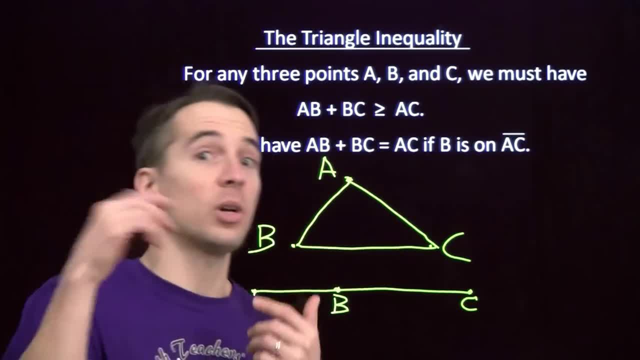 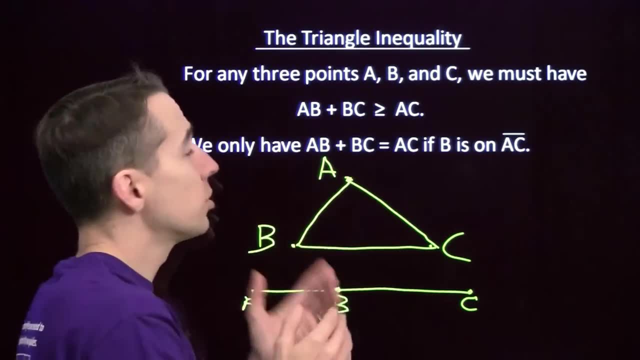 get a number that's greater than the third. 5 plus 6 is greater than 7,. 5 plus 7 is greater than 6,. 6 plus 7 is greater than 5.. That means I can make a triangle with the side lengths 5, 6, and 7..